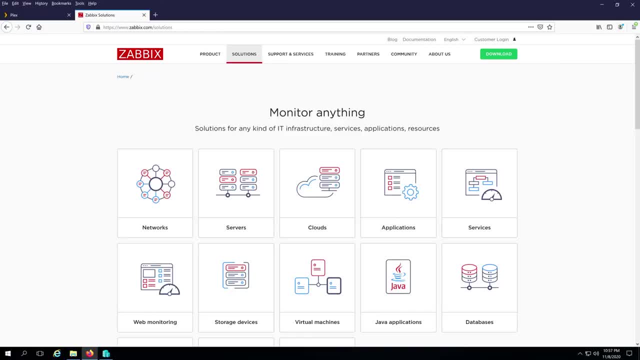 What's up everybody? In this video, I'm going to show you how to monitor your network for free. For this video tutorial, I'm going to be using Zabbix. I'm going to show you how to download, install and configure Zabbix. With Zabbix, you can monitor all kinds of networking equipment. 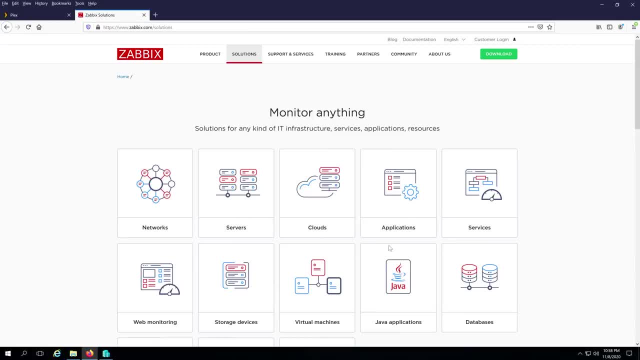 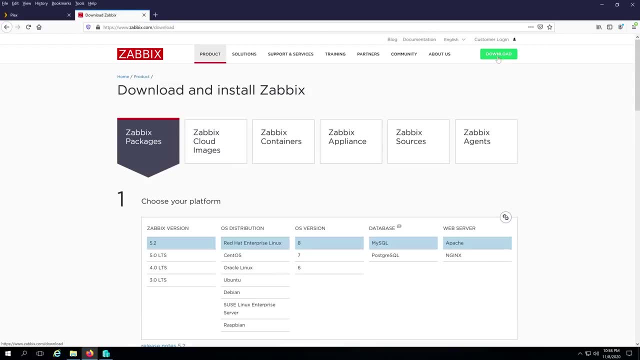 servers, application services and etc. You can monitor a lot of stuff with Zabbix. So here's first thing we need to do. We need to click on download and I will put link in the description below. Once we get to the download, you can install Zabbix on Linux, OSs or what I'm gonna do. 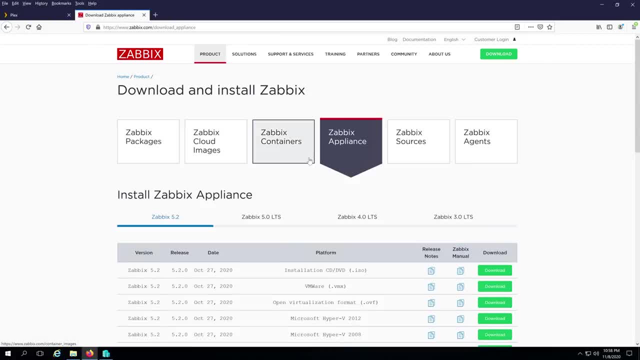 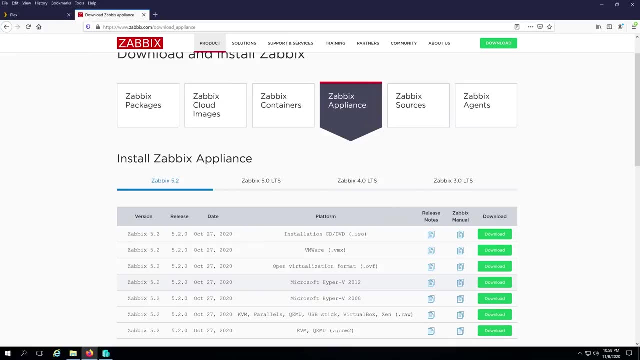 I'm gonna actually click on Zabbix appliance. I'm gonna still install a Zabbix on my virtual machine and you can use for that VirtualBox or Hyper-V or VMware, But for this video tutorial I'm going to be using Hyper-V. But instead of downloading Hyper-V 2012 right here, I'm just going to download. 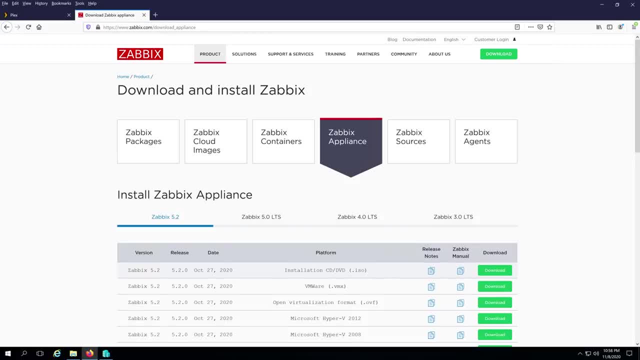 the installation. This is going to be online installation. So if you are going to be installing on something else besides virtual machine, make sure your system is connected to the internet. So what I'm going to do, I'm going to click on download right here and then I'm going to save this file Once the 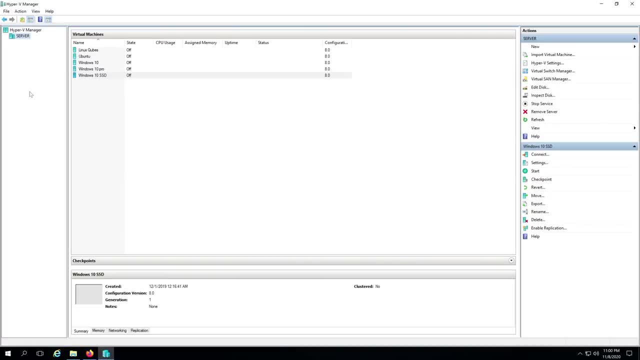 download is complete, I'm going to bring up my Hyper-V and in here I'm going to create virtual machine, really quick And right here. I'm going to choose image file and I'm going to navigate to my downloads, because that's where I'm going to be downloading. 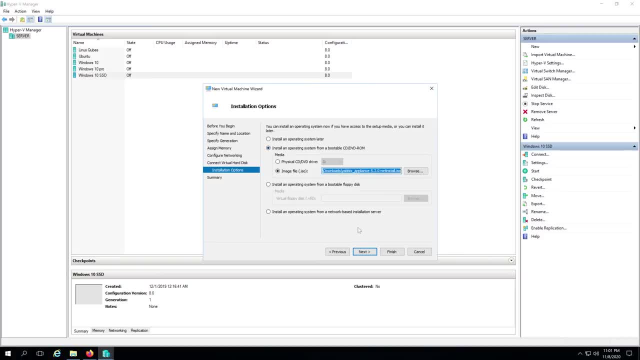 That's the application, the one I just downloaded. I'm going to click on open and I'm going to click on next. I'll click on finish. Okay, now virtual machine is created. What I'm going to do? I'm going to click. 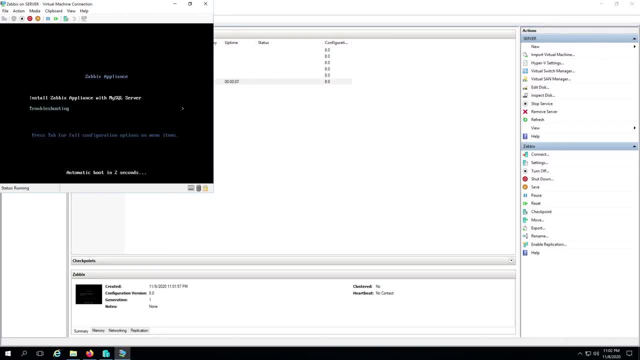 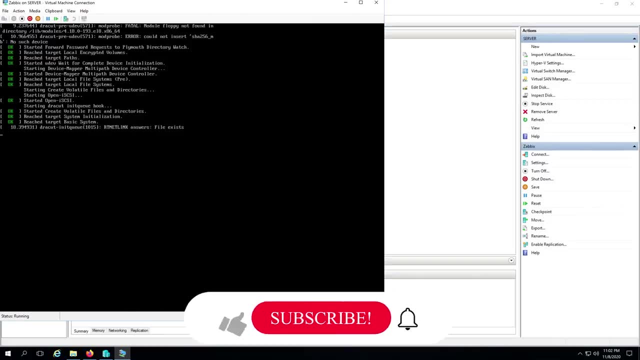 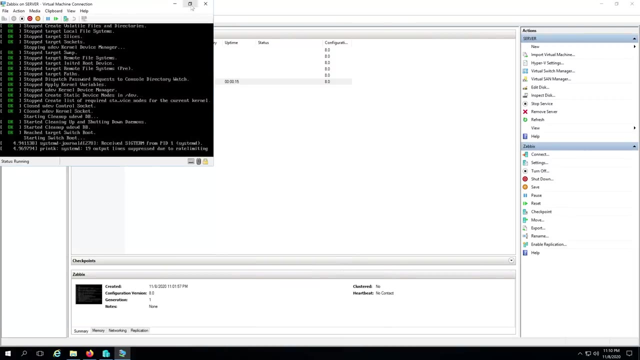 start and I'm going to click connect And in here we need to click uninstall Zabbix application. and now it's going to start installing the Zabbix. Once your system is done installing, what we need to do? we need to log in here within the virtual 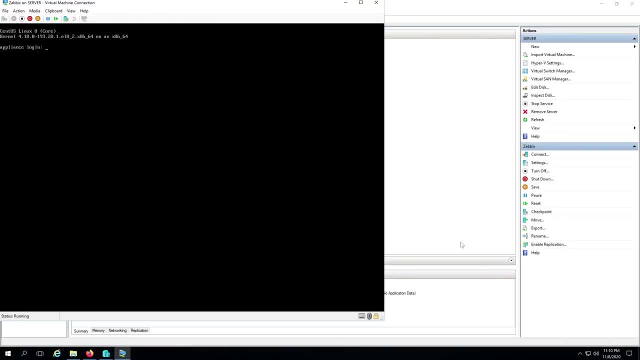 machine. We need to use our default credentials and the username is going to be root and password is going to be Zabbix, And then press enter And right here, once you log in, what we need to do we need to type IP address, and then we're going to type the IP address, and then we're going to type. 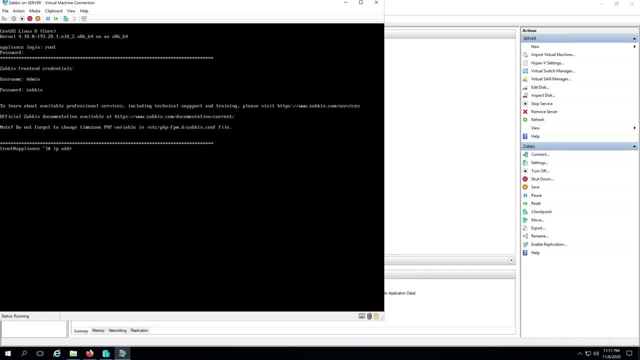 the password, and then we're going to type the password, Addr, and then show, and then press enter. So now this is going to show us the IP address of Zabbix. So here's what we need to do. We need to right now. we need to open our internet browser and 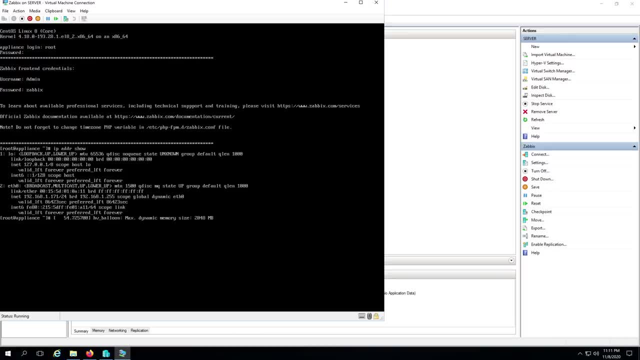 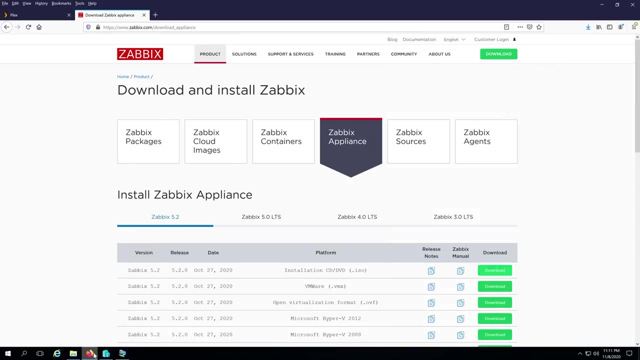 we need to type the IP address that we got. It's the IP address of the Zabbix server is right here, 192.168.1.172, and the username and password is going to be admin and password is Zabbix. So now we open our internet browser and right here I'm going to type 192.168.1.171 and I'm going to 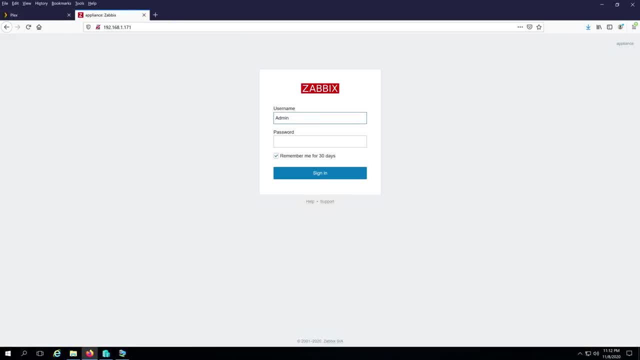 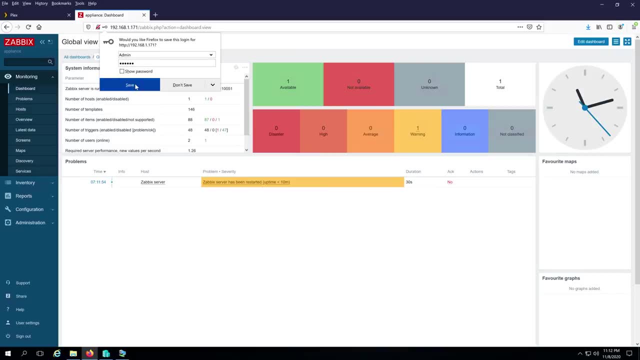 press enter and right here, username, admin, and then password is Zabbix, And then I'm going to click on sign in and my save password. for now, That's it. You have successfully installed Zabbix. So here's what we need to do. We need to add couple hosts. So what I'm going to do, I'm going to add a switch. 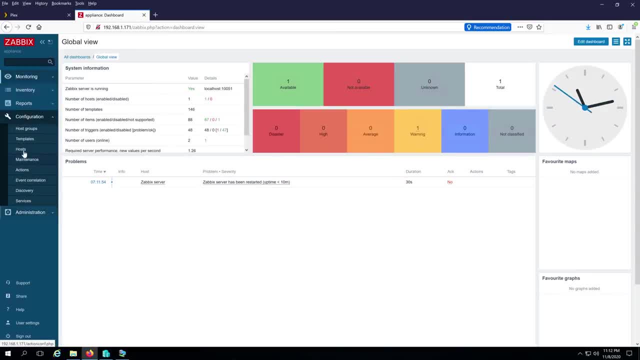 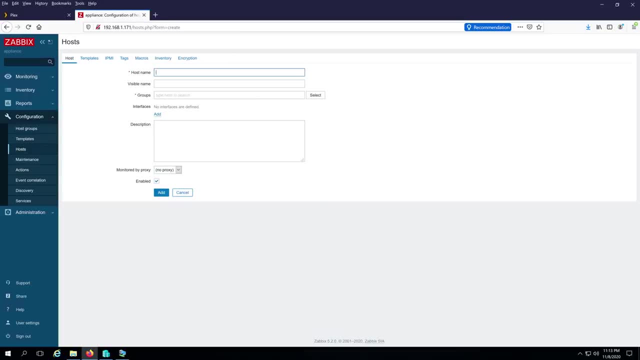 so what we need to do, we need to click on the configuration and then right here, we need to click on hosts, and in here we need to click on create host and right here we need to type- I'm just going to name it- switch, and then for a group, we need to select and right here we need to choose. 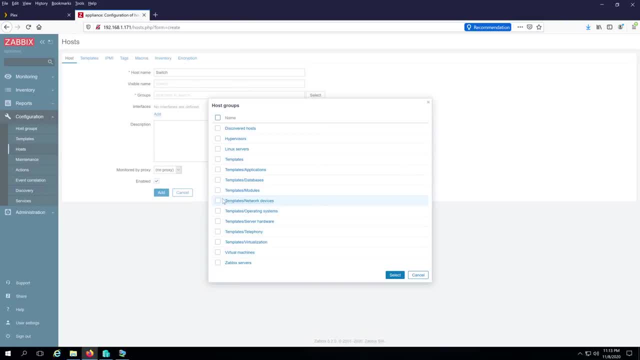 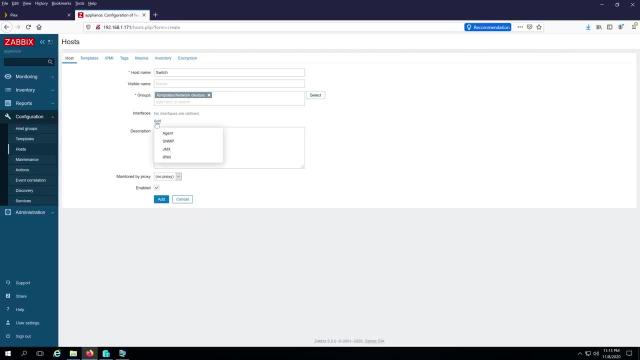 what this is and since it's networking device, I'm just going to use templates- networking device and then I'll click on select. Right here I'm going to click add. What I'm going to be doing, I'm going to be using SNMP and right here I need to type the IP address of my switch. it's 192.168.1.15. 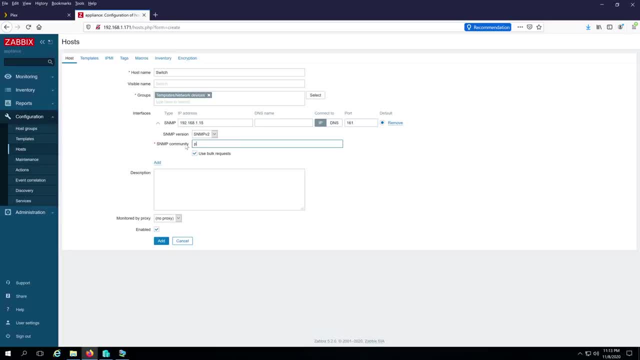 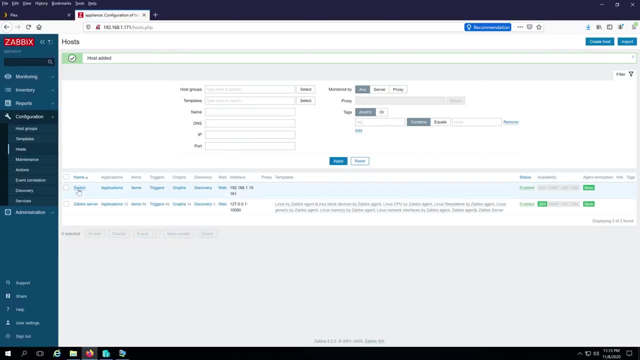 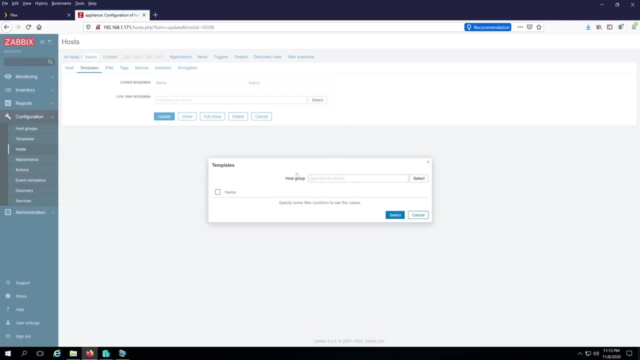 and right here for community string, I created password- Your could be something else- and then we need to click on add, Then we need to click on switch one more time and right here we need to click on templates, and in here we need to link new template. we need to select and then 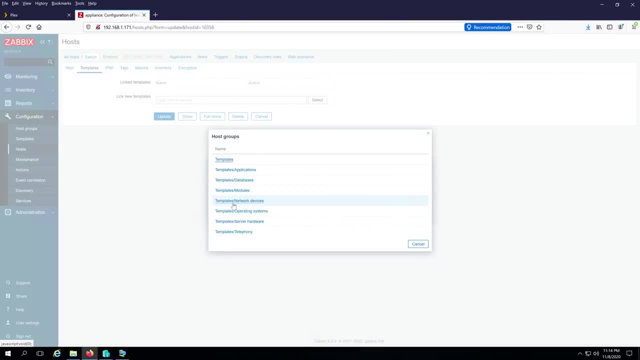 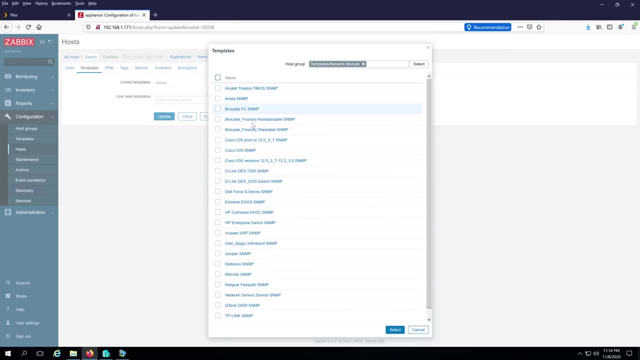 select one more time here and we're just going to choose network devices and in here I'm going to scroll down, since my switch- I'm using actron- is not in here I'm just gonna select network generic device, SNMP, and I'm gonna click select and I'm gonna click update and while it's connecting to my 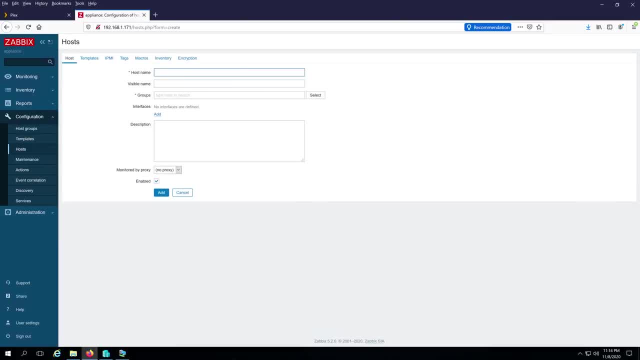 switch. I'm gonna create one more host, I'm gonna click on create and in here I'm gonna type server, I'm going to click on select and then I'm going to click operation system, because this is going to be server- and I'm going to click on select and then, in here, same thing, I'm going to click on add. 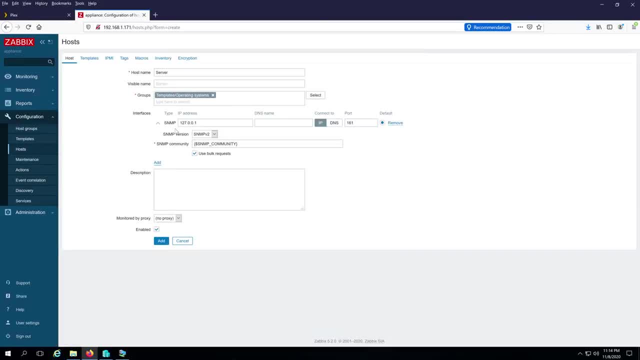 and I'm going to choose SNMP. So you have to make sure SNMP is enabled on your server or on any of your computers, the one that you're going to try to monitor. So first thing we need to do this is on server. we need to click on start and we need to type services, and then we need to choose services. 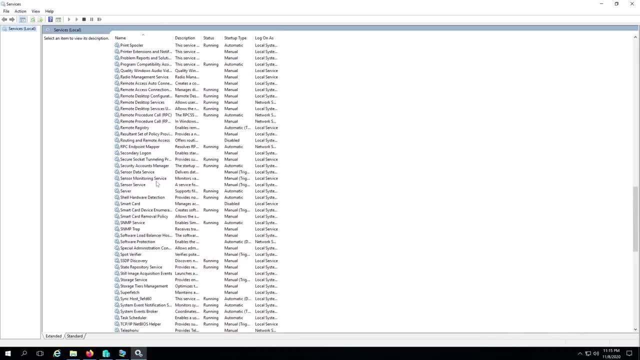 Once this is going to open up, we need to scroll down and we need to find SNMP service. We have to make sure it's here and we have to make sure it's running. and then what we need to do? we need to double click on it and then we need to click on agent. We have to make sure every service is. 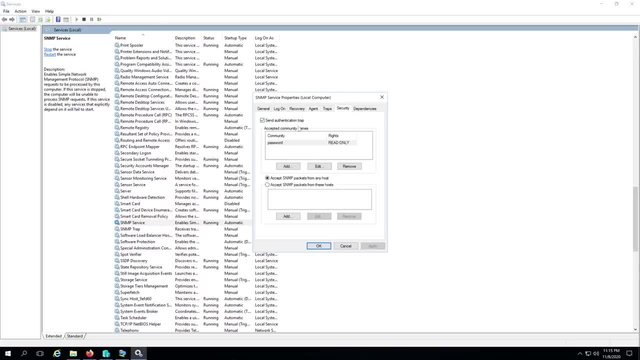 select here, and then we need to click on security. So, right here we need to create community string. so to do that, we need to click on create, just click on add, leave, read only and type whatever community stream would you like to type. I left password, so, and then in here we need to either accept SNMP packets from any host, or what? 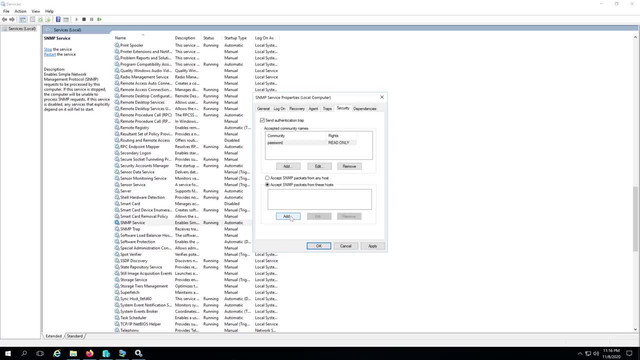 we can do. we can choose a specific host. if we choose that, then we need to type the IP address of Zabbix, and the IP address of Zabbix was 192.168.1.171 and then press add. if we do that, this is more secure way in case if somebody else is on your network, is trying to monitor or just fooling. 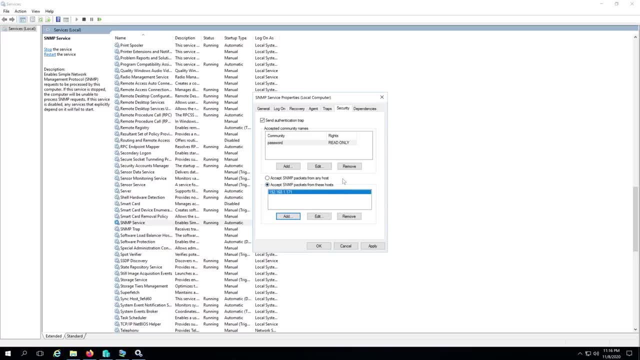 around, then you're not going to be able to pull any SNMP traffic and then we need to click apply and then ok. for example, if your SNMP service is not here, you see only SNMP traps. what you need to do? you need to install SNMP service. I'm going to link video in the description below how to install. 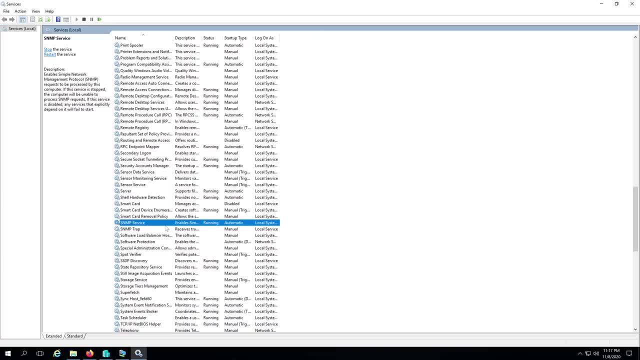 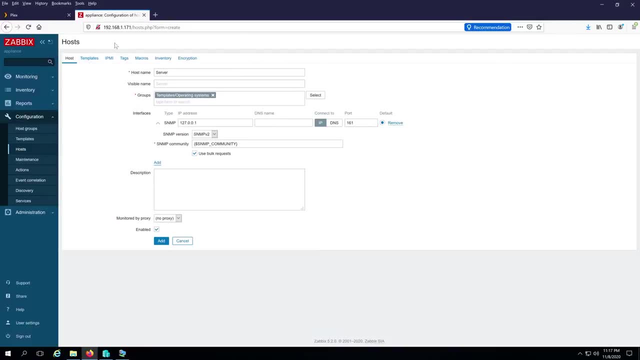 SNMP service, windows server and on windows 10.. once this is done, we need to close SNMP, we need to close services. and now we go back to Zabbix. so in here we need to type IP address of our server and again, if you don't know the IP address, you can click on start, type cmd and type ipconfig, and then 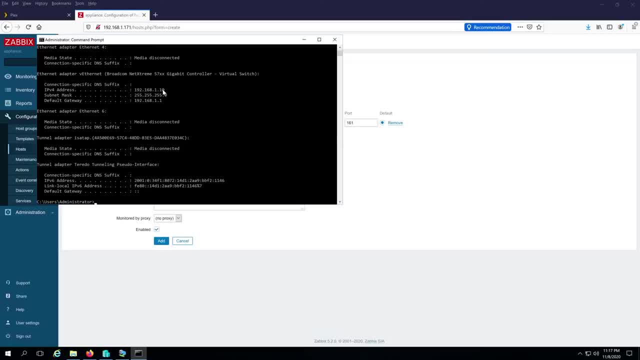 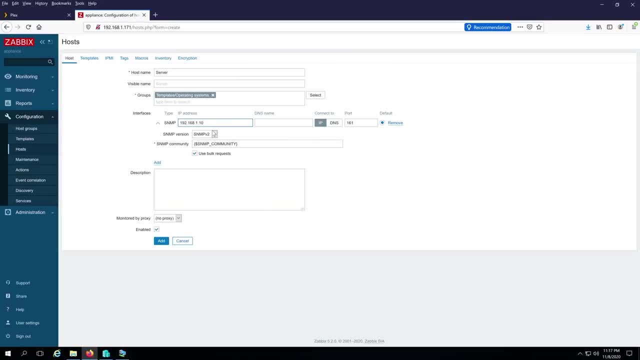 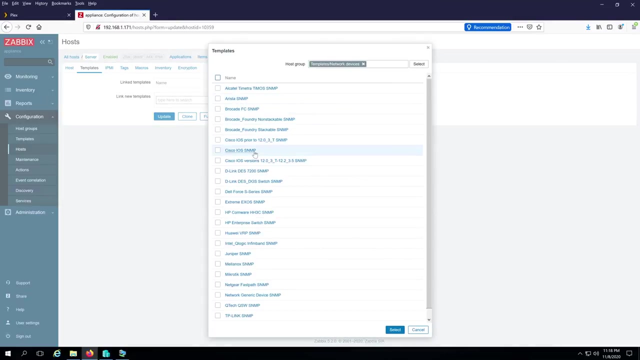 press enter and right here this is my IP address, my copy, and I'll paste right here. and then for SNMP I created password- yours could be something else- and then click on add and then once again click on server and then click on templates: select. right here we need to delete. 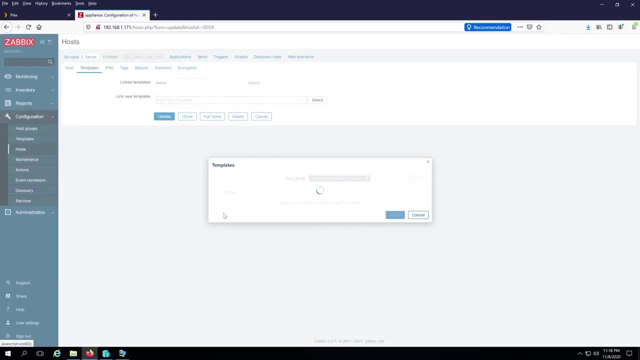 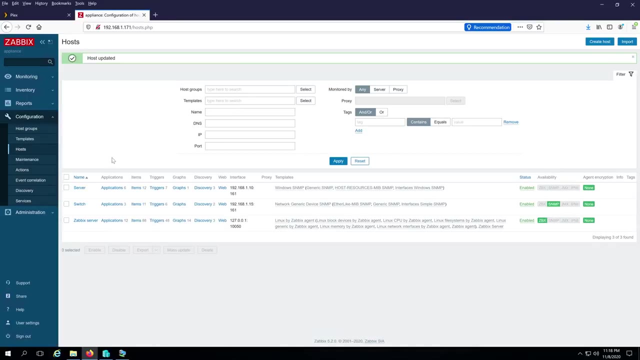 this and then click on select one more time, and this is going to be operation system, and right here we need to choose windows SNMP and you can choose all the other operation system that's out there available and then click on select and then click on update. okay, once this is done, you 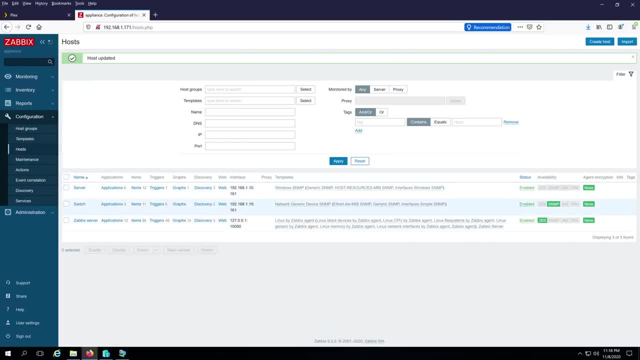 can see, my switch already established the connection with the SNMP and now we just have to wait until server is going to establish connection as well. once the connection is established, what we need to do- we also need to wait a little bit until it's going to detect. 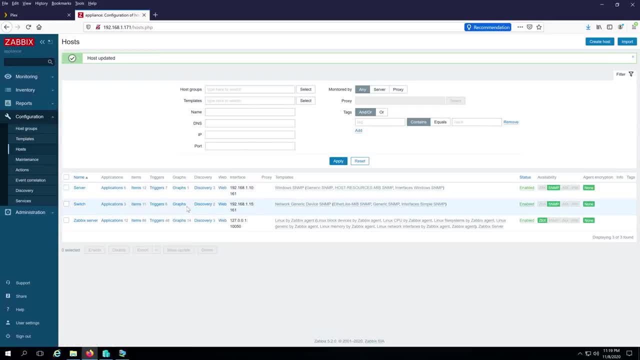 every graph that can be monitored. for example, on my switch I have 24 port switch. it's going to detect at least 24 or maybe even more graphs that we can recommend to do and monitor. and there's one more thing: what we need to do. we need to choose server or switch. 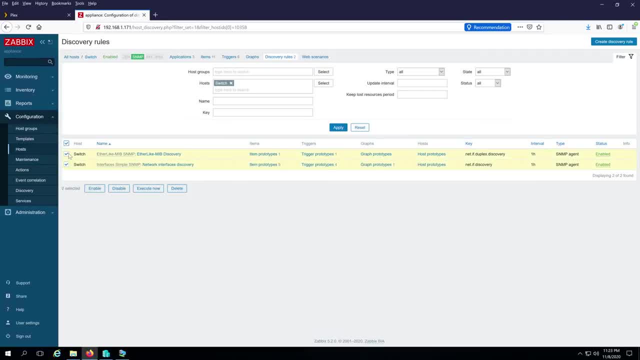 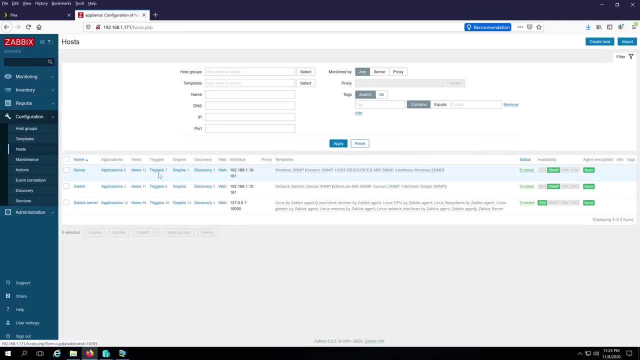 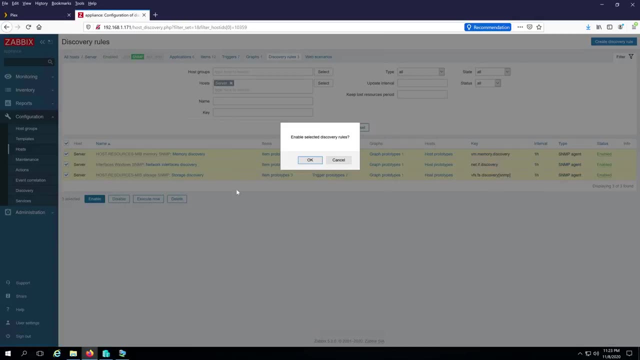 and then we need to click on discovery and right here we need to choose both of the switches and then we need to click execute now and then enable, and then same thing. go back to other hosts, click on on server, choose discovery and in here select all of the servers and then click enable. 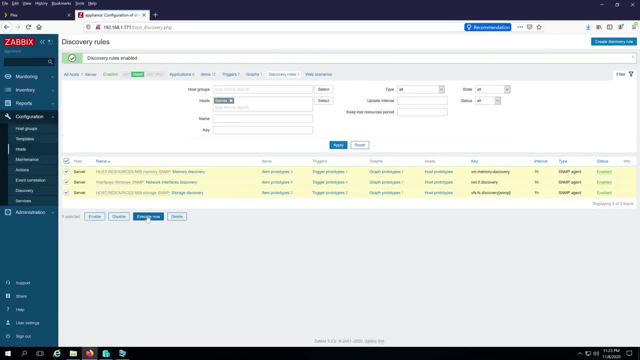 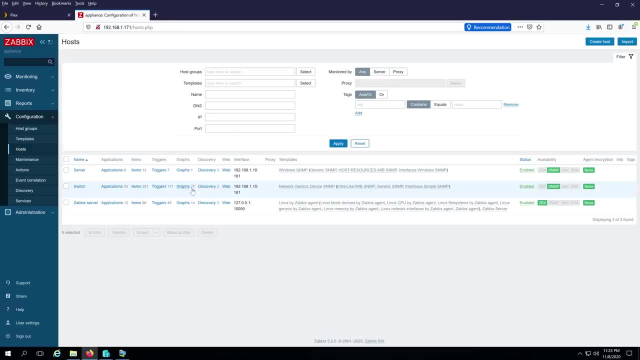 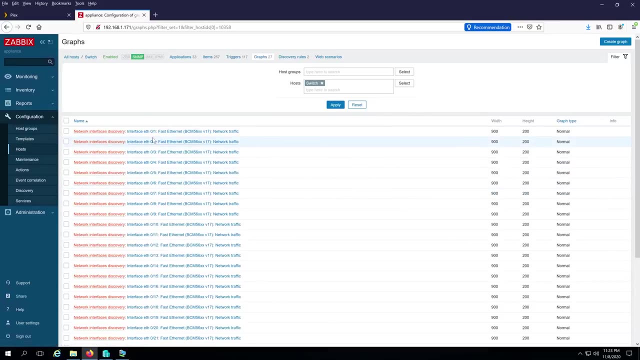 okay, and then execute now, select again, and then execute now, and then go back to host and once we try to discover, you can see the graph number is updating. so now what we need to do: we need to click on graph and right here we need to choose what exactly we would like to monitor. 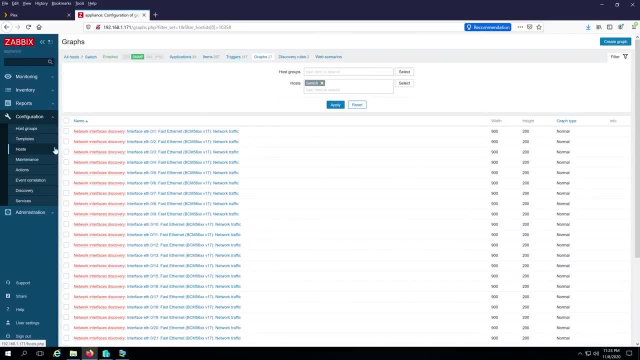 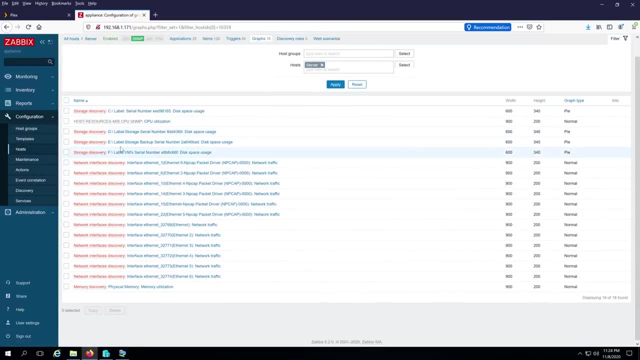 because it's going to create 27 graphs. i'm going to leave every single one of them and then in here, same thing for server is going to create 18 graphs. so now what we can do. we can click on monitoring tab and right here we need. 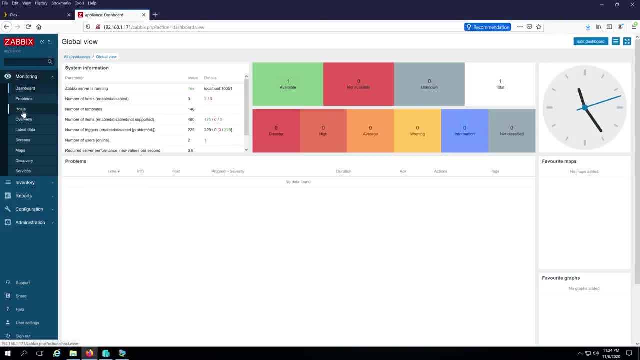 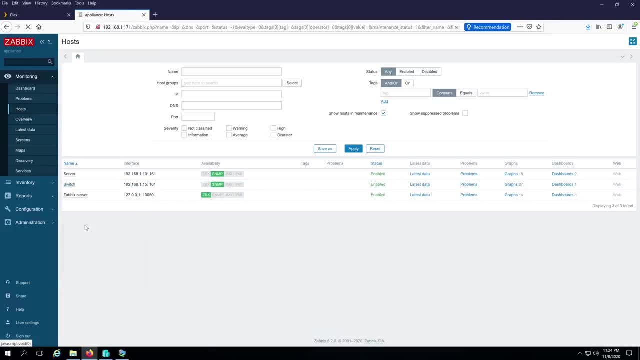 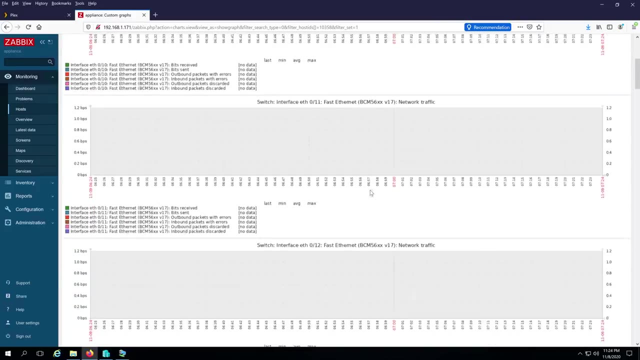 to click on dashboard and then we need to click on hosts. so in here in hosts, what we can do, we can choose switch and then click on graphs. and now it's going to show you graph for every possible interface that we can monitor so we can scroll down. you can see every single interface has a. 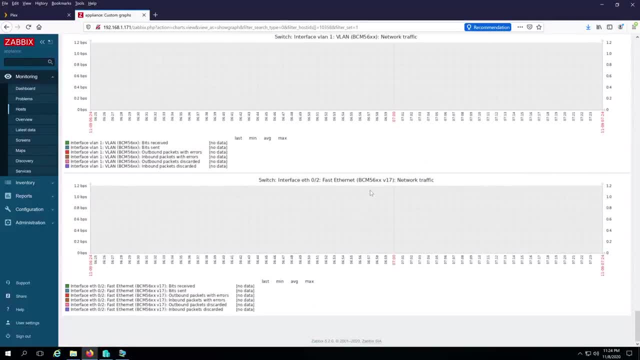 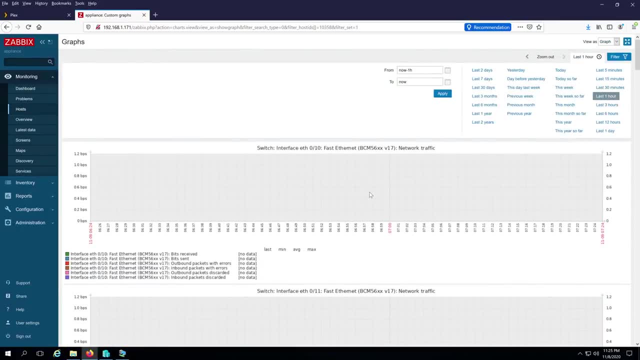 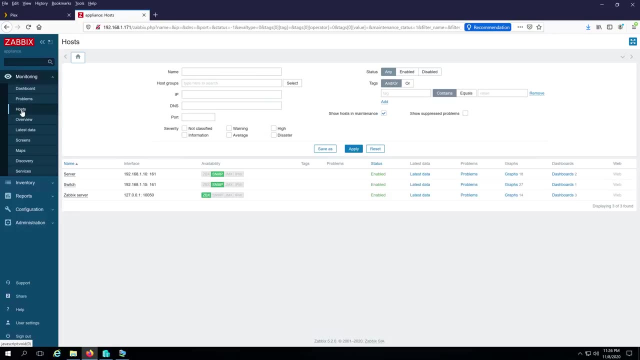 dedicated graph. i don't really have any data right now on it because there is nothing actually running on this switch. i'm going to try to transfer some files, so that way we're going to start seeing some data. then same thing. if we go back and we click on hosts, we can choose server and then 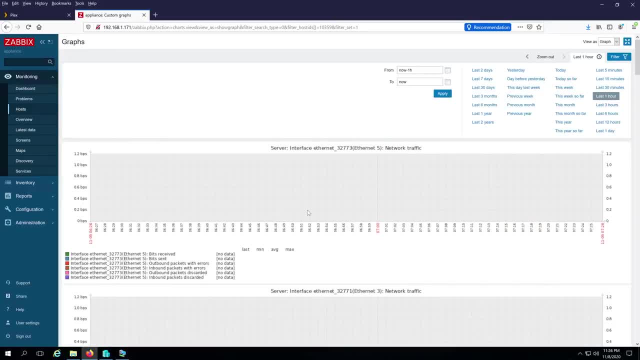 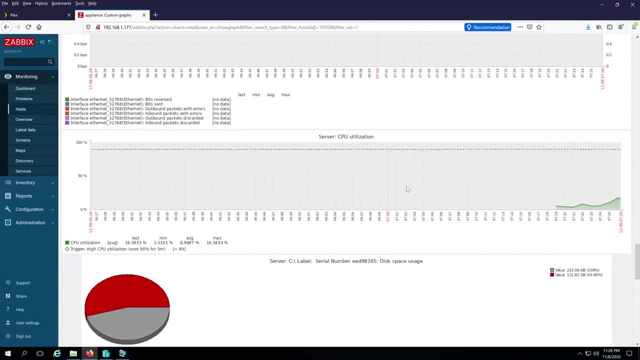 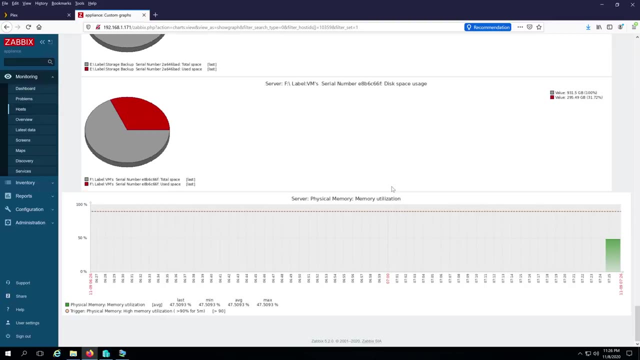 server. we can click on graphs. same thing. we're going to be able to get graph for every possible service that we can monitor and if you scroll down, you can see. if we click on dashboards, we can see how much data is being used. and on the right hand side, 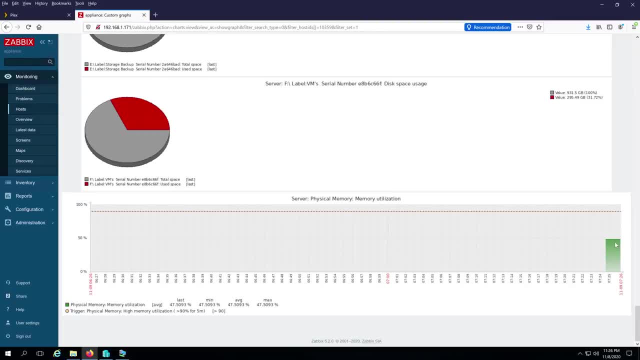 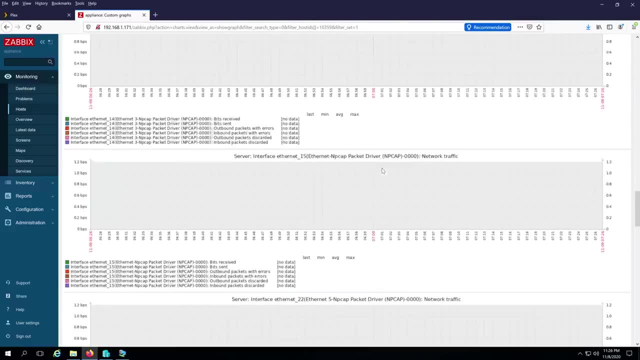 we can see all my cpu utilization. you can see all my hard drive, how much they're filled and everything else, and then physical memory. this is how much isn't used right now and if we're going to leave it running for a little bit, we're going to start getting a lot more data actually on here. 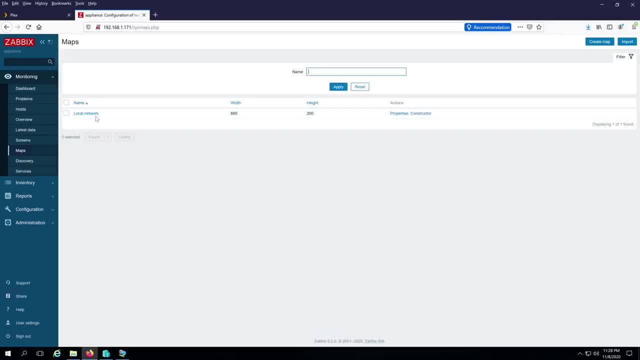 so then, what we can do, we can click on dashboard. we're going to create and we're going to add a map here, so we need to navigate to maps one, but I'm just going to use default one and in here, what we need to do, we're going to need to. 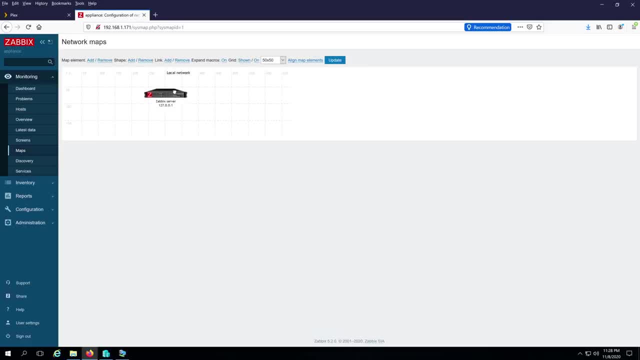 click on edit map. So what I'm going to do? I'm going to move this server right in the center. this is my Zabbix server, the one that is running, and you can change the settings just by clicking on the server itself. you can change all the settings over here. I'm going to click close. 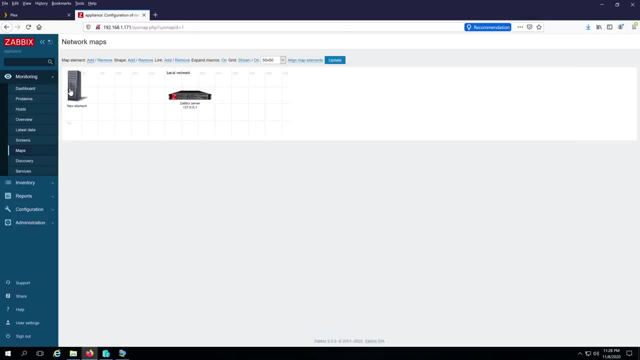 so what I'm going to do, I'm going to click on map element and it's going to add a new element, so I'm going to leave it right here, for example, and I'm going to change this element. I'm going to name it as a switch. so I'm going to click on image, I'm going to click on host and in here, 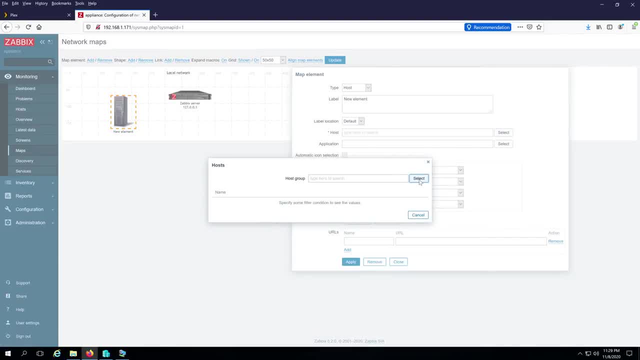 I'm going to click on select, I'm going to close this and I'm going to choose a switch, or from networking devices. this is from the template that we're going to use, because this is my switch and I'm going to choose switch, so it's going to bring up my switch. so, right here we need to change the. 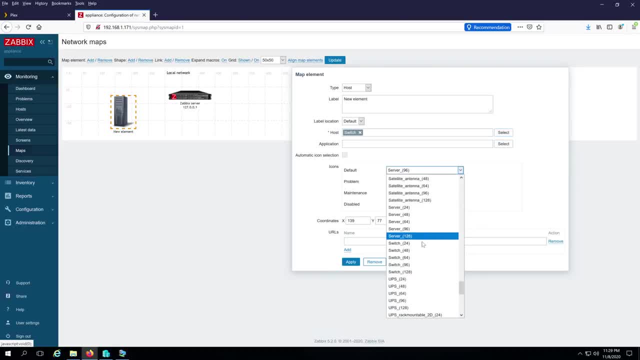 icon from the default from the server. I'm going to change to a switch and I'm going to change to a switch and I'm going to use 64 and I'm going to click on apply and then close. so then, what I'm going to do, I'm going to highlight both of the devices and I'm going to add a link between: 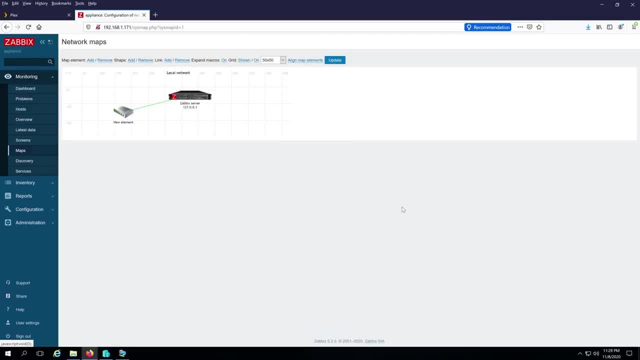 them and then I'm going to apply and then close. so then I'm going to add one more element, I'm going to move it right here and this is going to be my server. I'm going to click on it in images and I'm going to close this template and I'm going to click on select again and I'm going to choose. 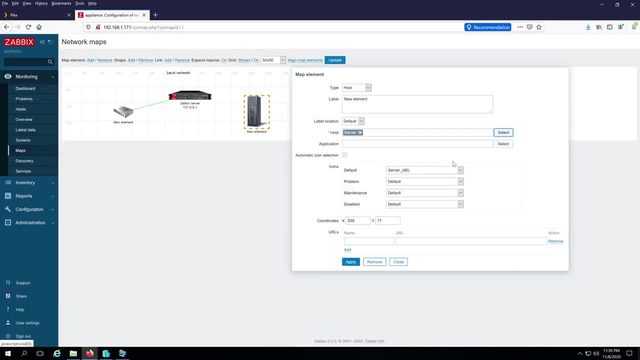 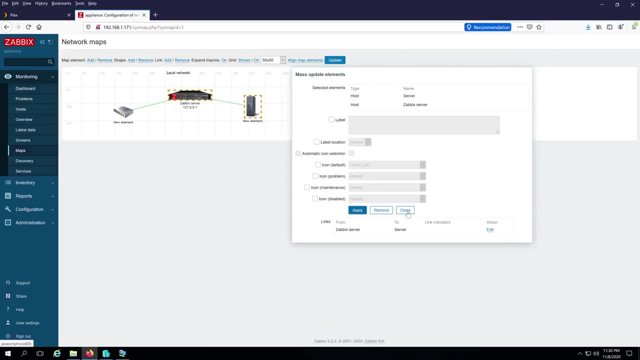 operation system, because this is my server and I'm going to click on server and in here I'm going to change this to 64, so it's not going to be that big, and then I'm going to click on apply and close. same thing. I'm going to highlight this and I'm going to add a link and then I'm going to apply. 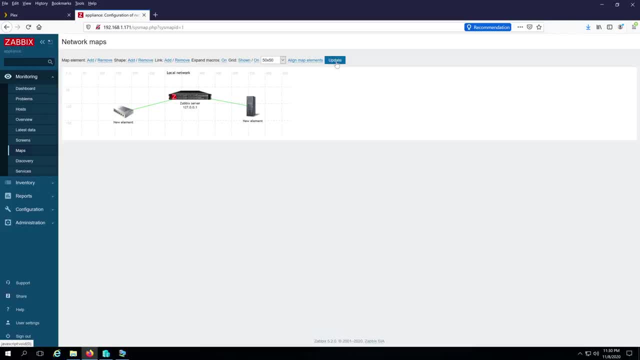 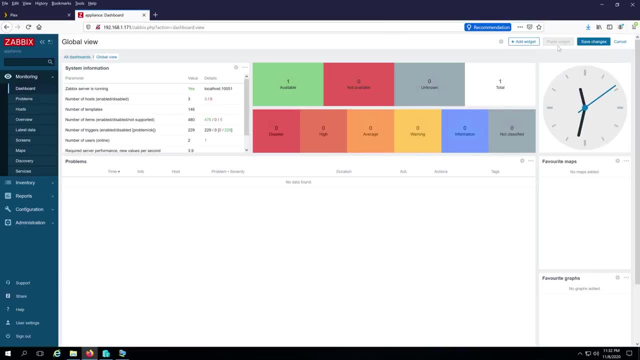 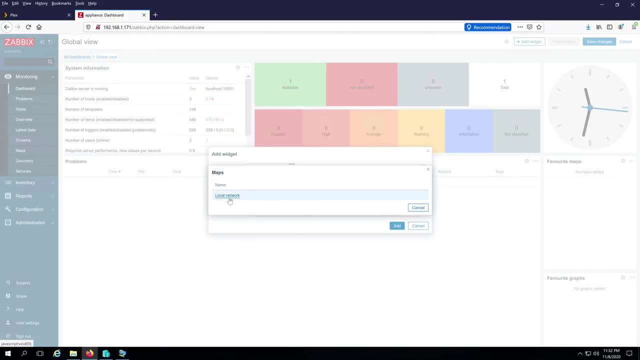 and I'm going to click close. once the map is complete, we can click on update and then click OK and go back to dashboard and in here we need to click on edit dashboard and then add a widget and right here we need to choose map and then in here we need to select and we need to click local. 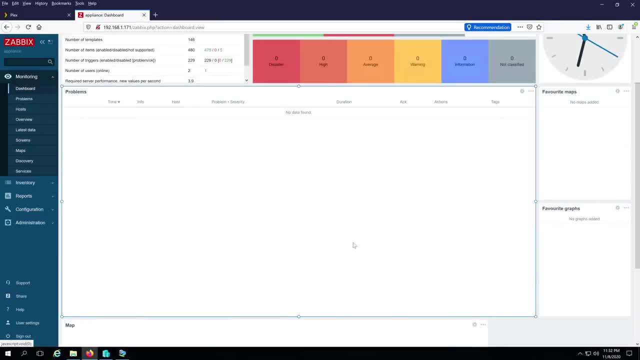 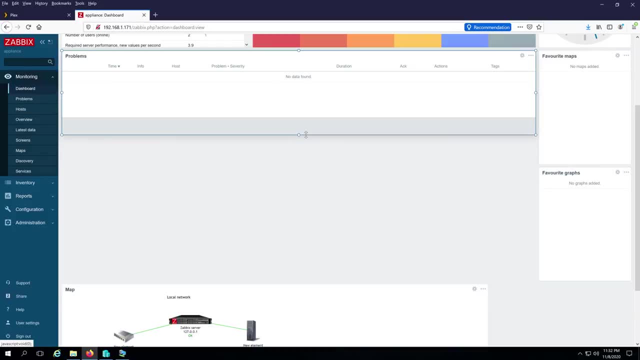 network, because that's the only one we have, and then we need to click on add, so it's going to add this map over here. so what I'm going to do, I'm going to select this, I'm going to shrink it down and then I'm going to move this map and I'm going to put it right here. 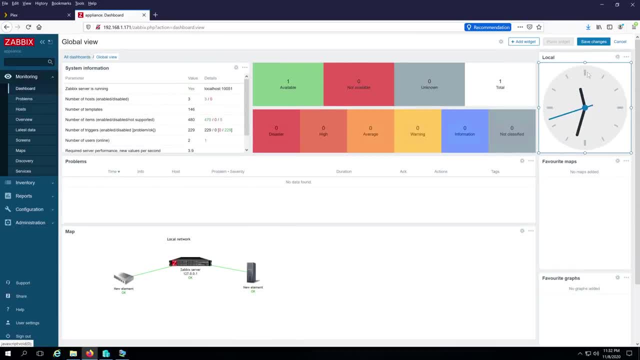 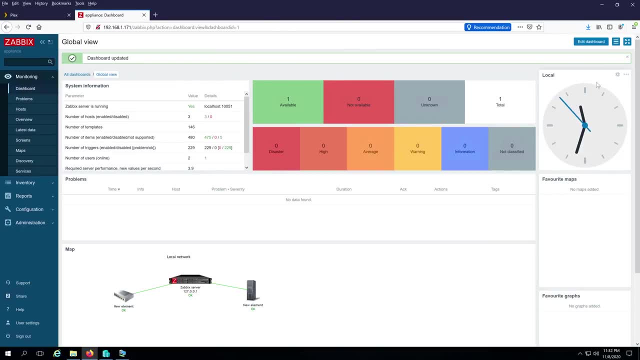 and then, once you're done moving stuff around, what we need to do? we need to save changes once the changes are saved. so here's what we got here. we have the clock, we can add more widgets, but we got two main tabs. we got problems here, so if there's any problem, it's going to be detected.